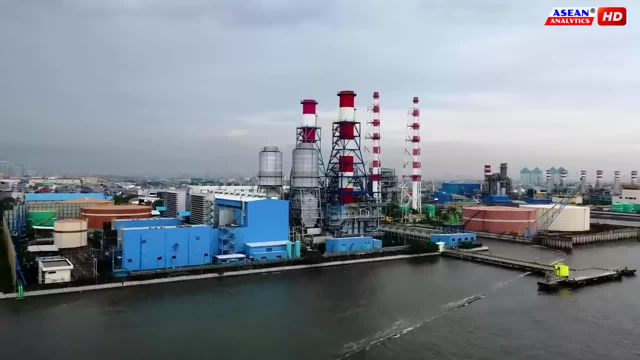 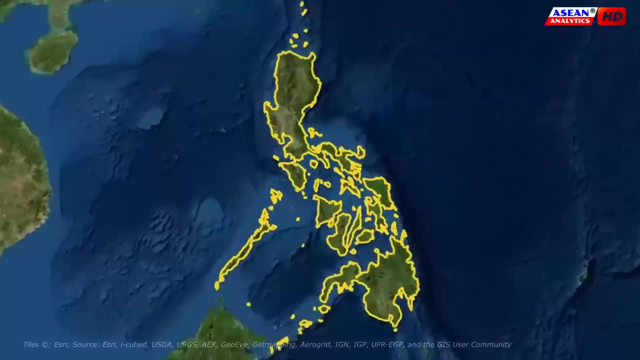 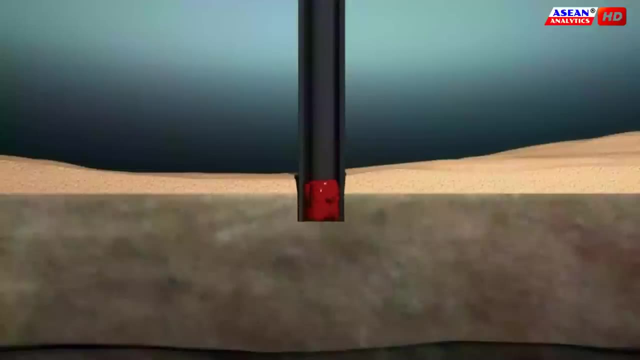 provide an answer to the unabated rise of gasoline prices. almost every week, The Philippines is sitting on a mountain of gold. Within the country's 200-mile exclusive economic zone are potentially recoverable hydrocarbon deposits Worth an estimated of more than $26.3. trillion, More than enough to develop the country into an advanced economy. One of the reasons why the Philippines is unable to materialize its oil reserve is the security challenges and geopolitical disputes. The vast oil reserves of the Philippines are in various parts of the archipelago. 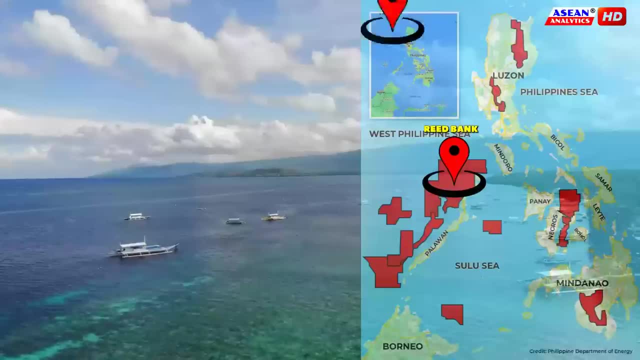 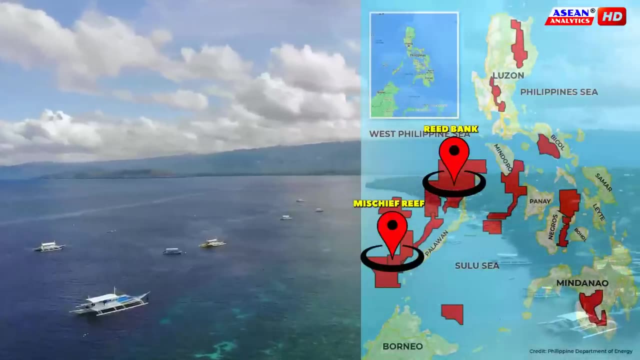 specifically the Reed Bank, the largest of them all, And the Mischief Reef in Kalayan Island Group, as well as the other basins, are located within or in the surrounding disputed Spratly Islands, A group of islands and associated reefs banks. 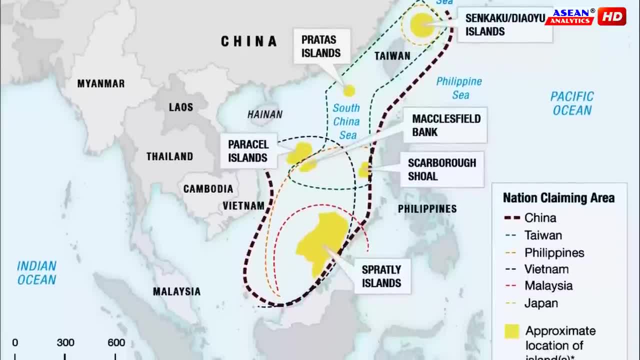 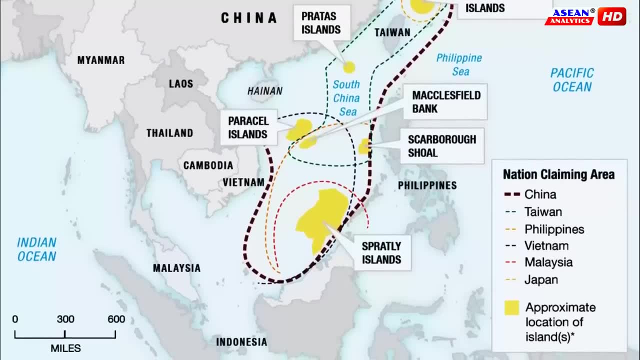 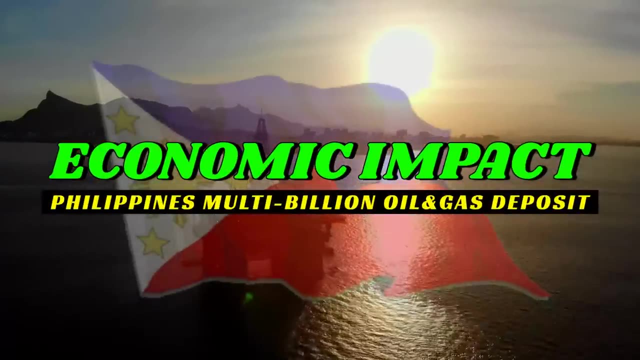 and quays located in the South China Sea are subject to a territorial dispute between China, the Philippines, Taiwan, Malaysia, Vietnam and Brunei. No oil prices have a significant impact on the economy, but soluble oil production in the Philippines may lead to a drop in production. And oil prices in the Philippines do not appear to be a major problem, though. In addition to US oil prices, the country's oil prices have not changed since the Star Wars days In the Philippines. Taiwan, Malaysia, Vietnam and Brunei are two of the main major global industries in Pei Sng. 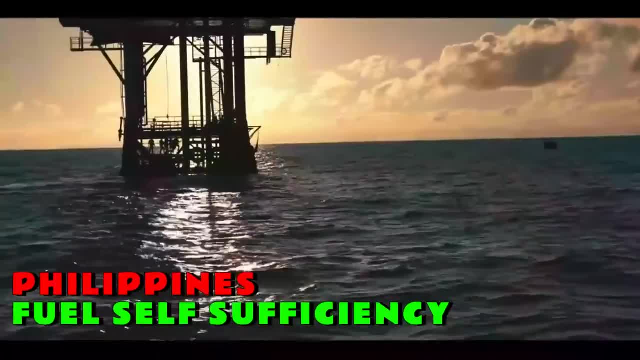 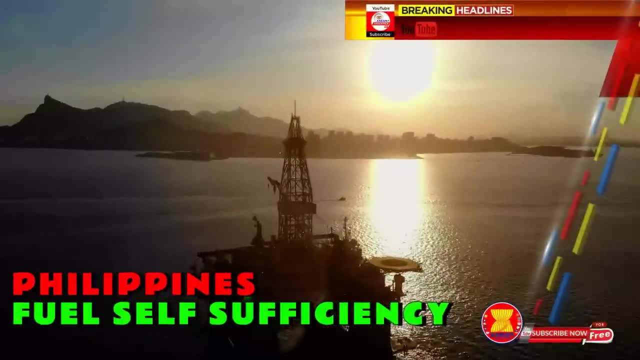 Their oil prices are expected to drop significantly, and they are not expected to drop under prepared oil prices. carbon fuel self-sufficiency remains a pipe dream for the government for decades. Though it's not a question of where and how much the deposit is, it is a question of when it will be fully. 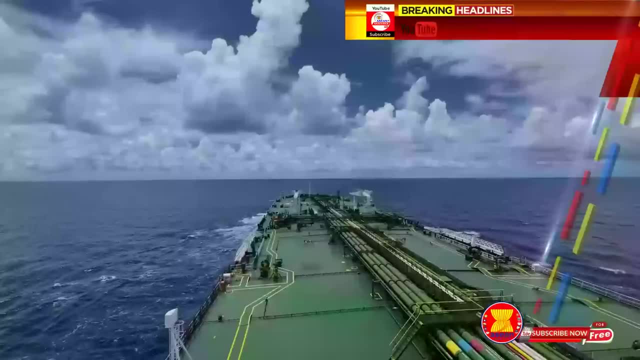 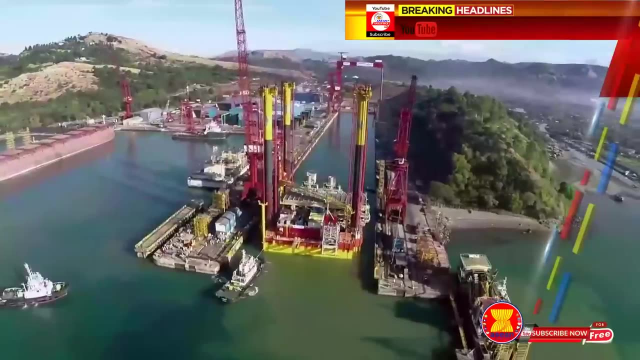 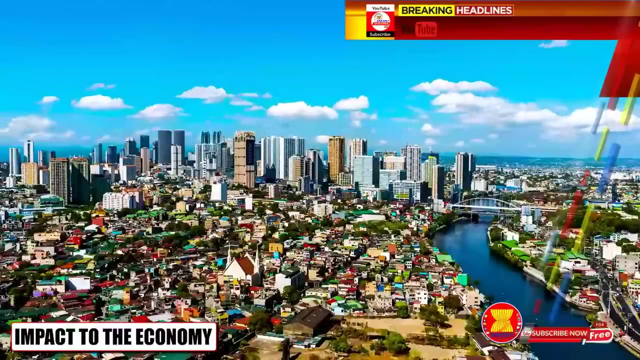 materialized When commercial production began. the Philippines would not have to import expensive oil. In fact, the country would be an exporter of oil products and simultaneously provide an answer to the unabated rise of gasoline prices when the supply chain is disrupted. In addition, 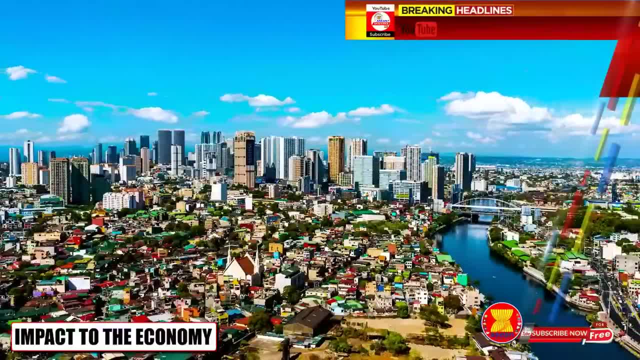 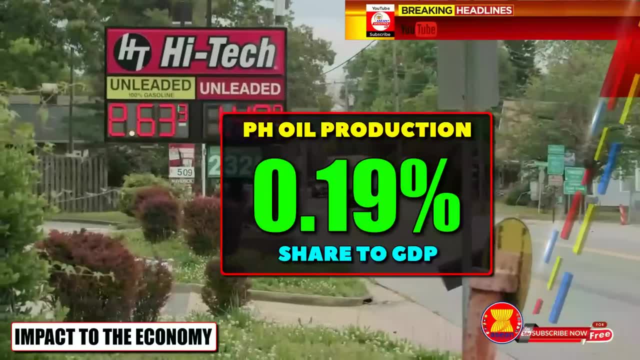 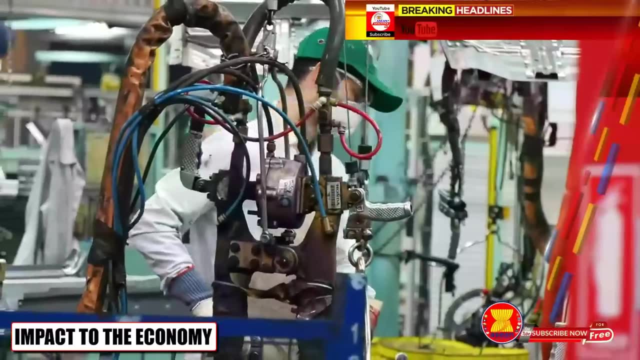 it will have a huge impact on the Philippines' economy. According to the Philippine Statistics Authority, the share of the oil industry, particularly non-renewable resources, been only 0.19% of the gross domestic product GDP for the last 20 years. This industry is also one. 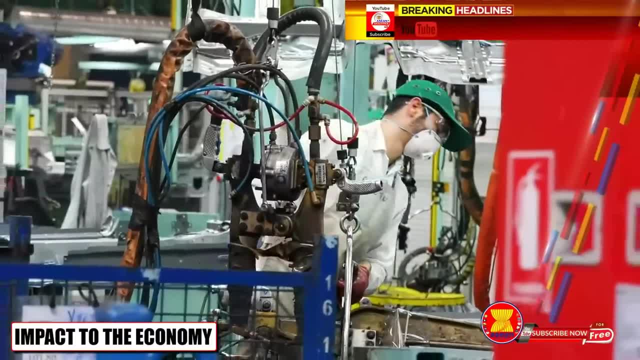 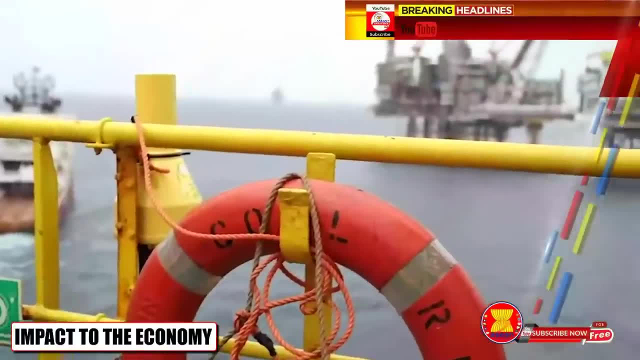 of the most significant contributors to manufacturing costs. Once commercial production started, granting that the surveys are accurate, it could potentially provide a significant portion of the Philippine economy. The Philippine economy is a very important part of the Philippine economy. The Philippine economy is a very important part of the Philippine economy. 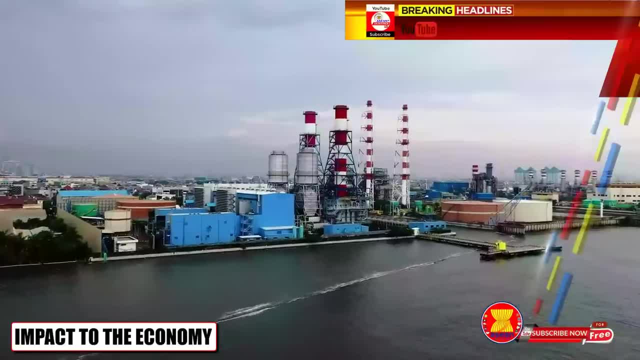 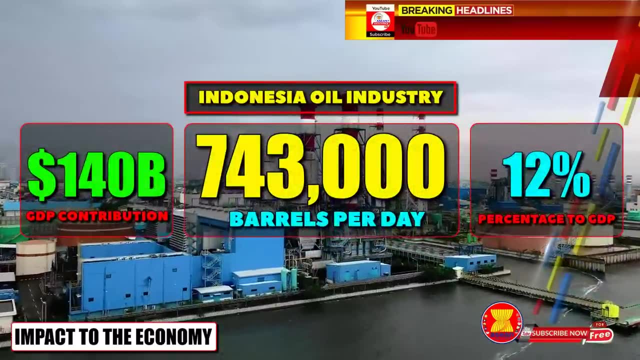 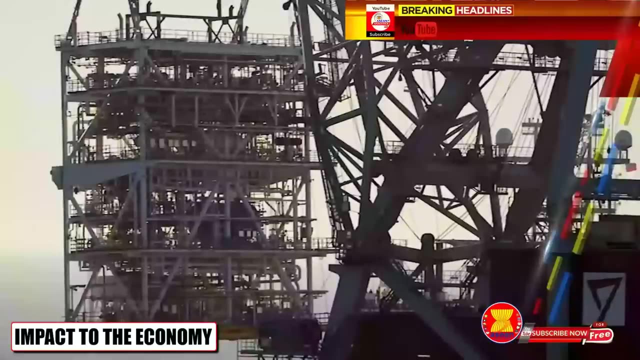 In comparison to Indonesia, the region's biggest oil producer, with a production of about 743,000 barrels per day in 2020, contributed at least $140 billion annually, or about 12% of its economy, If the Philippines can produce at least the same level, or a bit higher, than Indonesia. 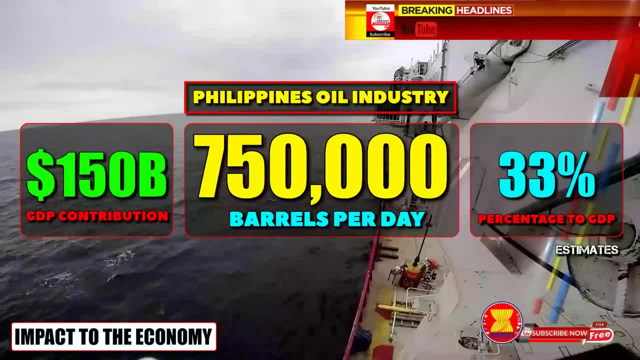 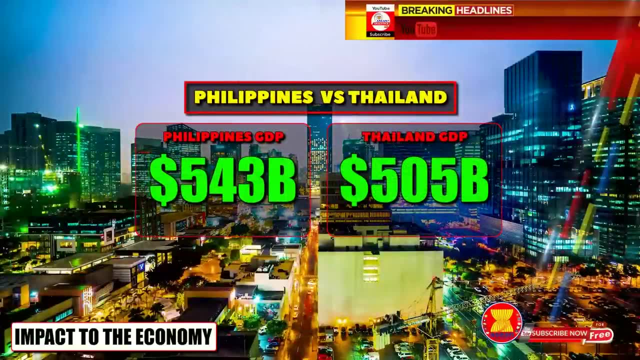 the country's oil and gas industry can contribute at least $150 billion or more annually to the country's economy. The Philippine economy is a very important part of the Philippine economy, Making the Philippines the second biggest economy in the region, surpassing Thailand with a GDP. 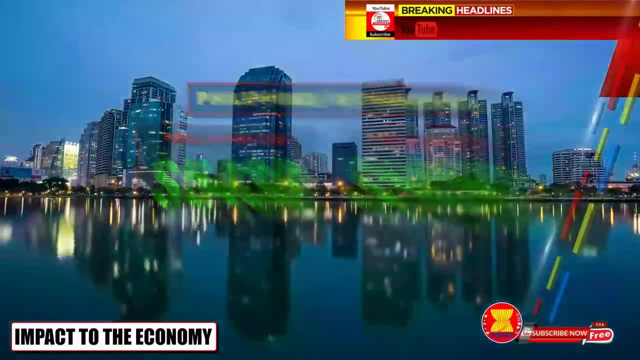 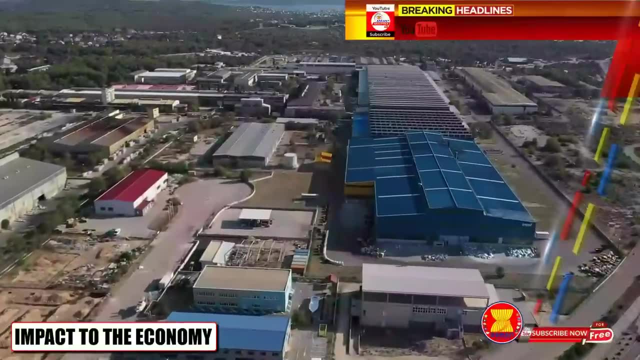 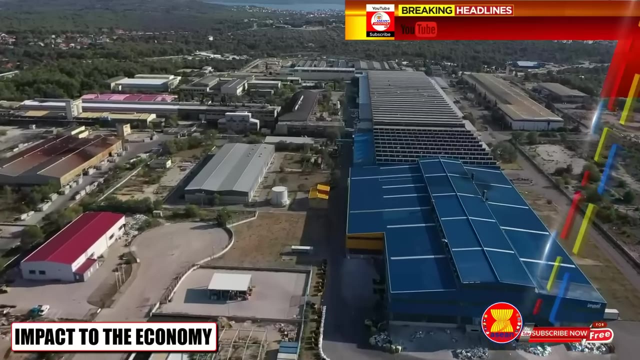 nominal of $505.9 billion. This will also enhance the competitive edge of the country in terms of manufacturing goods With a lower production cost. the Philippines can now compete with Vietnam and Indonesia, the region's cheapest producer of goods, Making the country an ideal alternative. 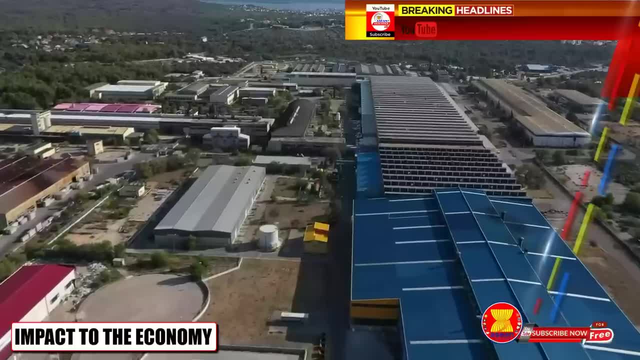 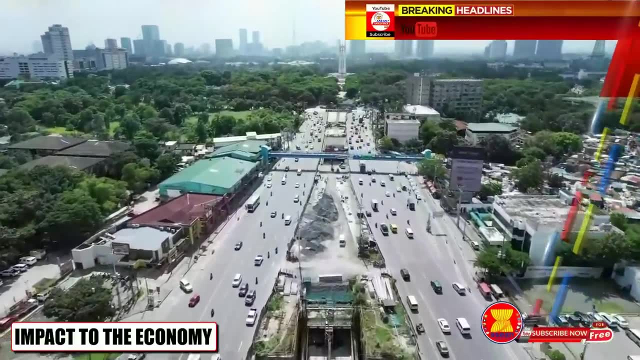 location for manufacturing hubs in Asia. Those increasing the overall production cost of the country's oil and gas industry can now compete with Vietnam and Indonesia. direct foreign investment in the country. In addition, transportation costs and other basic commodity prices will be now more economical. With locally produced oil means no more import cost. 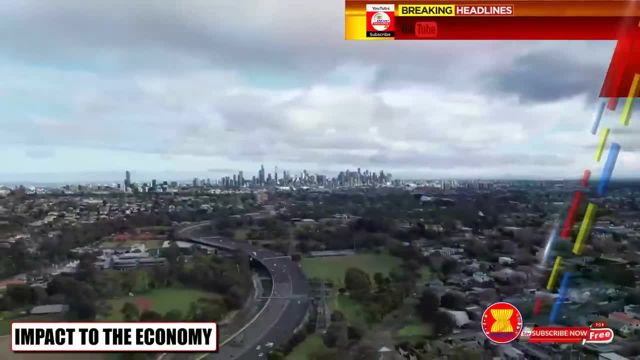 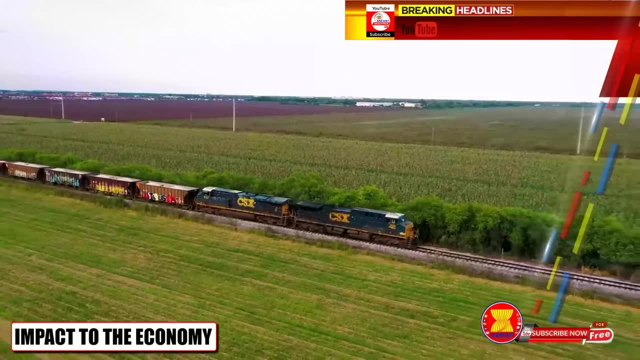 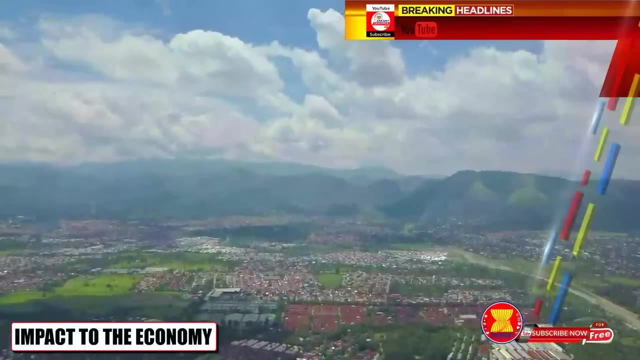 making petroleum products cheaper. In effect, transportation and other logistics will be cheaper, lowering the cost of basic commodities such as agricultural and other processed products. When commodity prices are low and even the household income remains unchanged, it means higher disposable income. In other words, a household's regular income would afford more amount of goods. 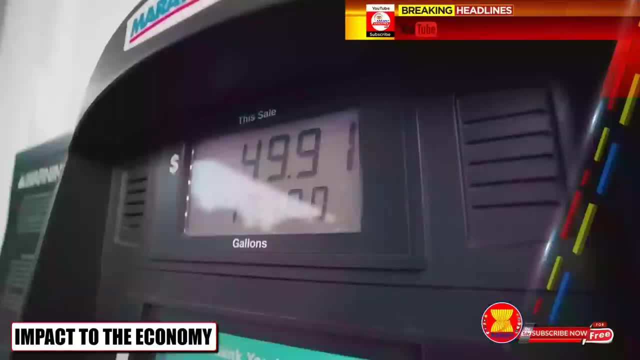 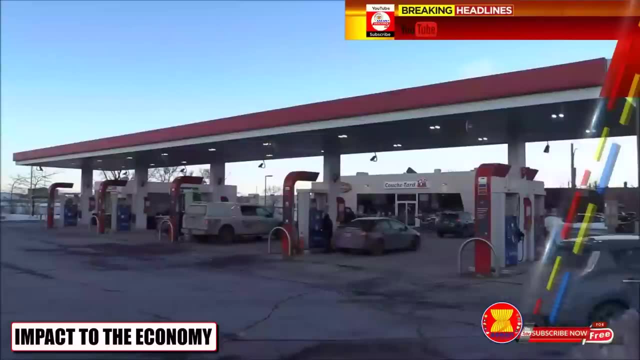 With these, inflation in the country will remain low. Currently, a 10% rise in oil prices could add 0.4 percentage points to Philippine inflation. To add, the Central Bank of the Philippines also sees the high oil prices to drive inflation as high as between 2% to 6%. This situation will 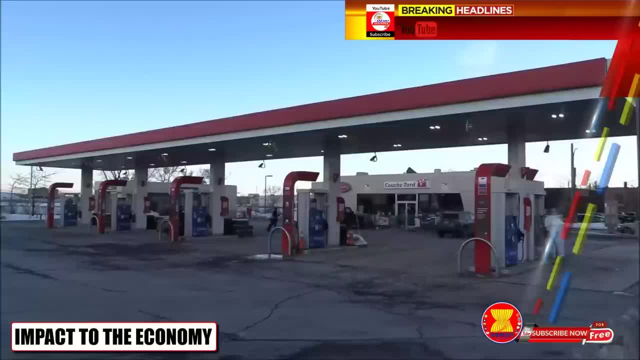 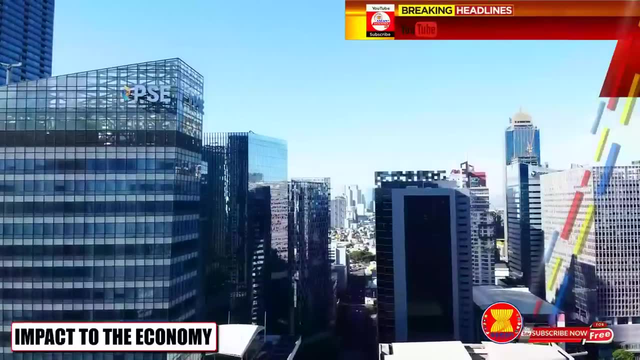 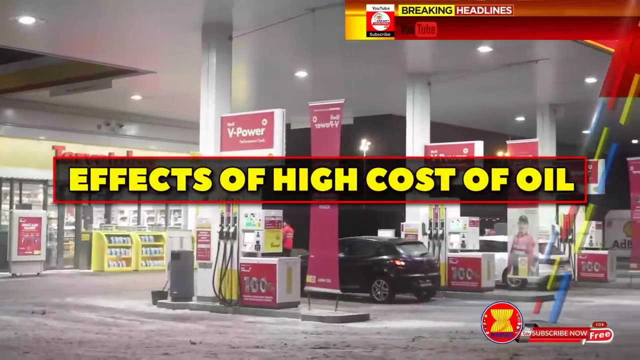 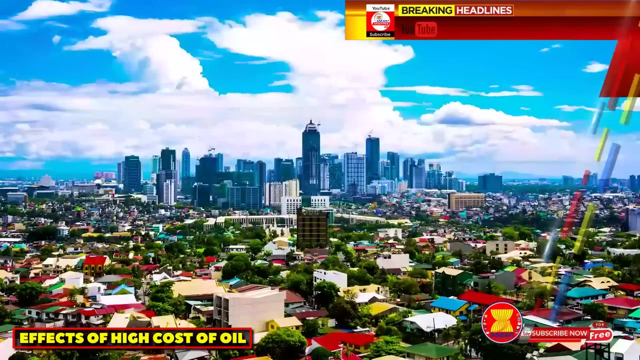 be diluted when the Philippines will produce domestic petroleum. Overall, these will enhance the private domestic consumption of Filipinos, which remains the main driver of the economy, accounting for 70% of the country's economy. In the long run, sustained oil price hikes can slow down the growth of an economy. 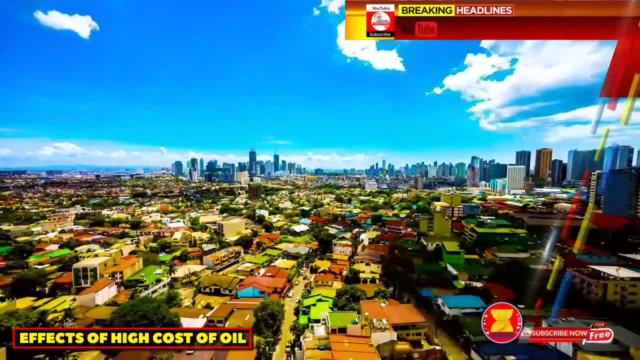 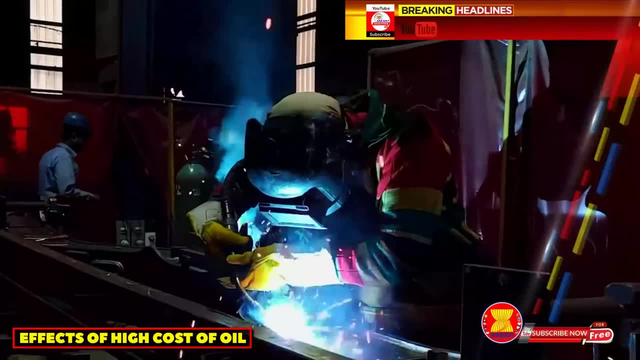 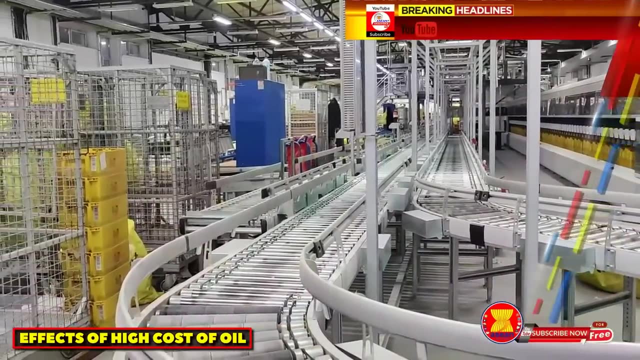 Like an ordinary household. the Philippine economy in general is also up for a rough ride. Production, Production, transportation and manufacturing costs are also driven up by high oil prices. While consumers are still not shouldering these costs, producers cannot cushion them for long. 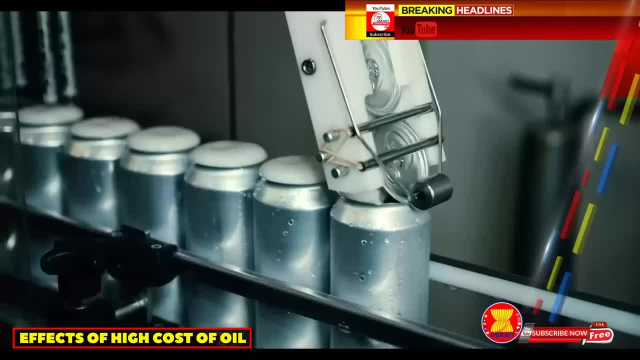 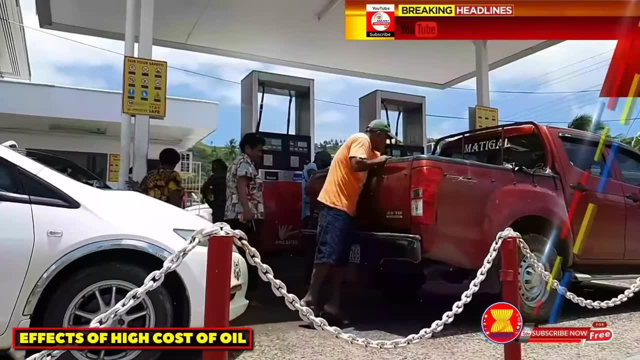 As a result, these will be passed down to the consumers, increasing the overall prices of goods and services and causing inflation. The impact of increasing oil prices does not limit to an economic slowdown and high inflation. it will also affect investments, With an expected slowdown of. 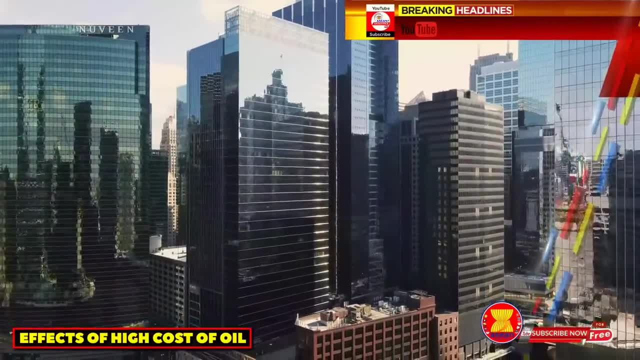 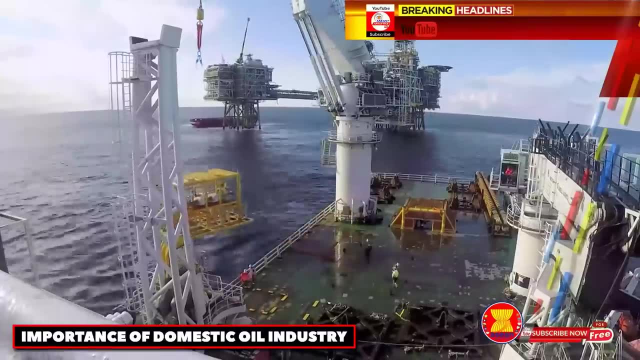 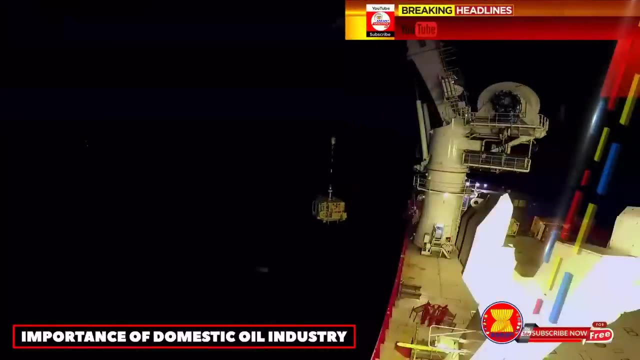 economic growth and rising production costs, companies also adjust their revenue expectations. The significance of producing domestic petroleum products has a material effect on the overall economy. The oil and gas industry will only not support the creation of a domestic job, but, most importantly, provides lower energy costs for consumers and ensures the energy security of the country. The affordability and accessibility of domestically produced oil and gas are infusing hundreds of millions of dollars of competition. In the process of our own production industry, we lose the ability to produce additiveness to our domestic production. In the process of our own production industry, we lose the ability to produce additiveness to our domestic production. 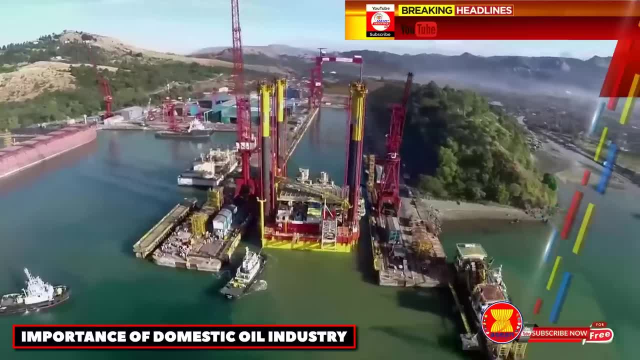 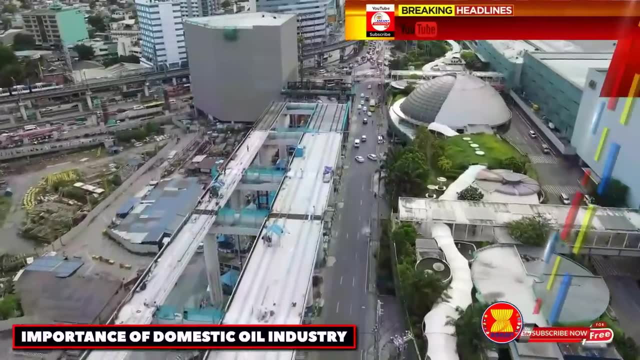 schwierig mankind classemakingier domestic products of oil and gas industry to diversify because companies softer increase consumption of oil and gas. that is, stove-soapan. oil and gas are infusing hundreds of billions of dollars into New Philippines manufacturing, supporting the development of new jobs, infrastructure and economic opportunity in communities throughout. 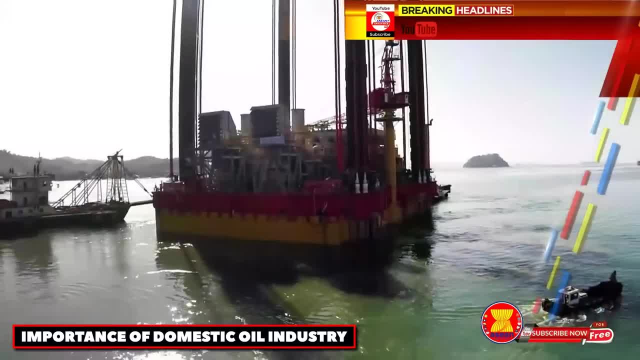 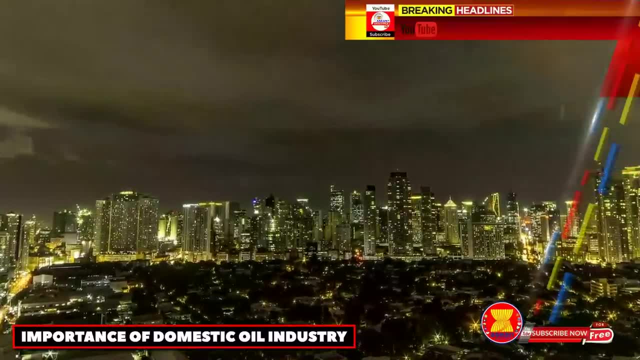 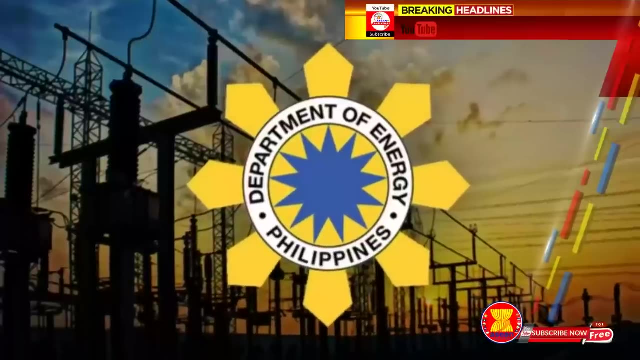 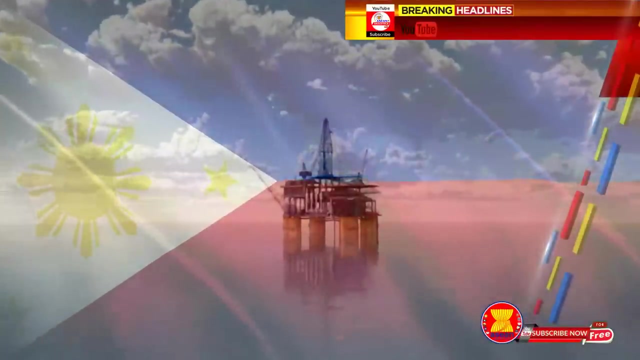 the country: Lower energy costs driven by more massive oil and gas supply, support private sector investment in the country and, further, by economic growth. The Philippines Department of Energy has outlined an overly ambitious two-fold agenda of attaining energy security and implementing power market reforms. By 2040, the Philippine oil and gas sector intends to increase reserves. 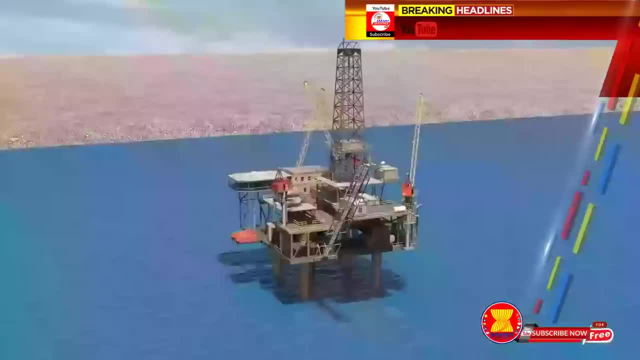 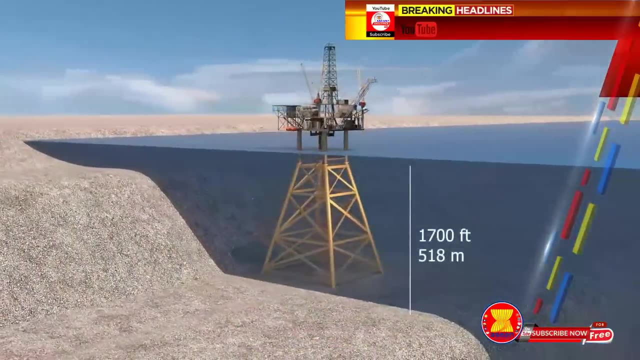 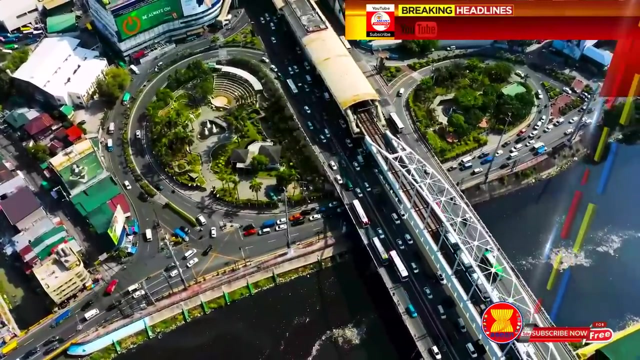 and production of local oil, gas and coal. improve downstream oil industry policies for the continuous supply of high-quality and quantity petroleum products. and establish an investment driven natural gas industry in the Philippines. The Philippines assumes that the population will increase from 110 million in 2020 to 148 million in 2023. Such plans are critical, as the country faces a loss of almost 30% of its fuel supply source, which will impact approximately 3,000 megawatts of generation in 2024. when the Malampaya natural gas fields are expected to be depleted, The nation needs to find a new source of energy. 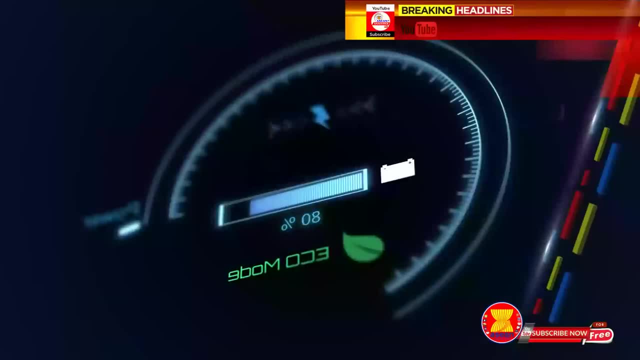 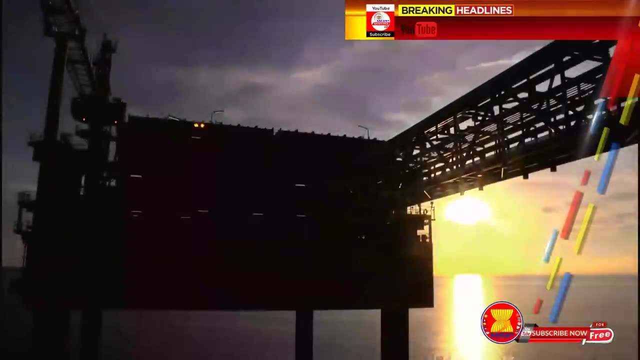 to compensate for this loss as it seeks to maintain its economic growth and support the country's infrastructure boom. The country has proven the presence of commercial quantities of hydrocarbons in the country's oil and gas industry. The country has proven the presence of commercial commodities in its territory, both onshore and offshore The industry. however, 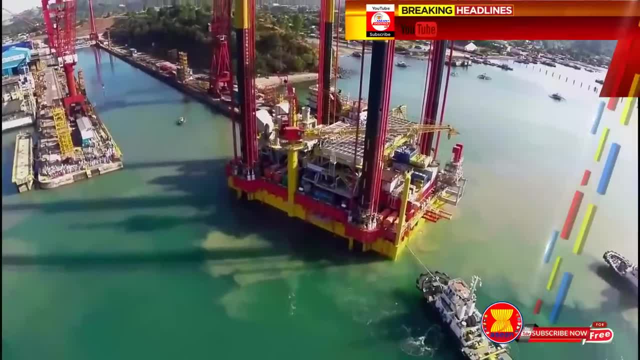 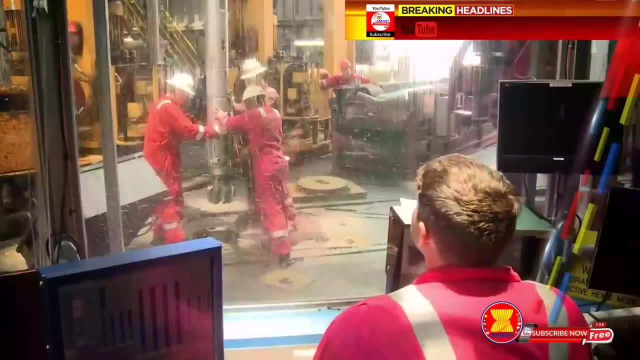 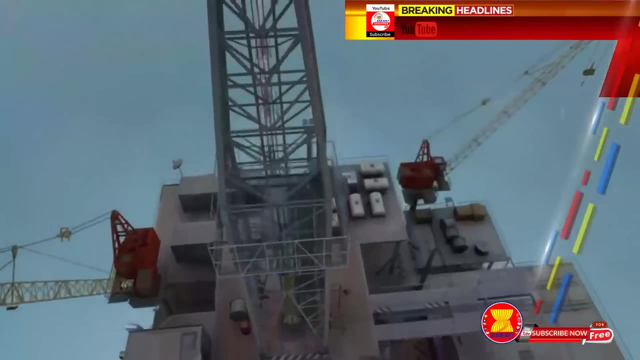 is underexplored and underfunded due to some security concerns. Since the 1970s, only a few wells had been drilled, supplying a small chunk of the domestic oil and gas demand. for its more than 110 million inhabitants, Total domestic production of petroleum and other liquids was: 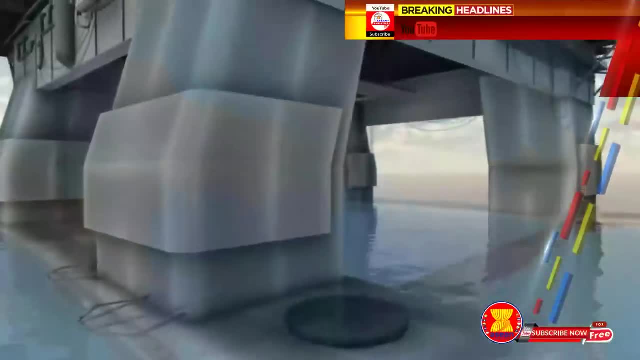 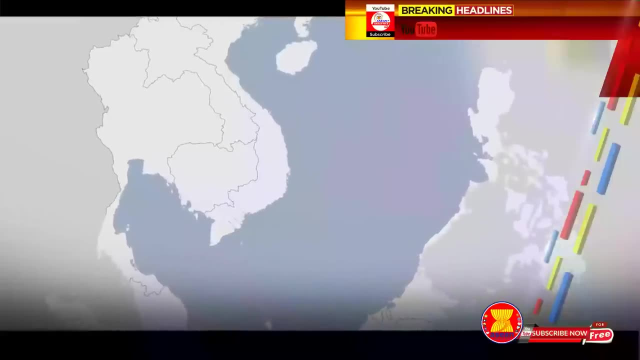 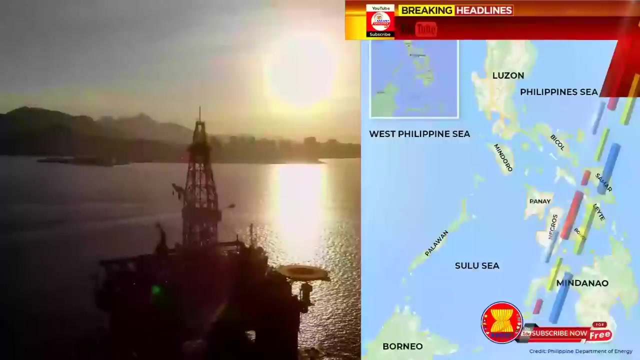 37,000 barrels per day, compared to the country's daily consumption of 474,000 barrels, according to the Ministry of Energy. Some of the oil and gas are found in the disputed Spratly chain of islands, where active oil fields are now supplying the rest of the country. Other prospective deposits are: 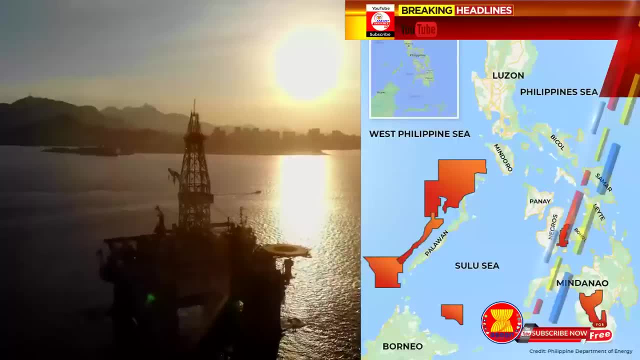 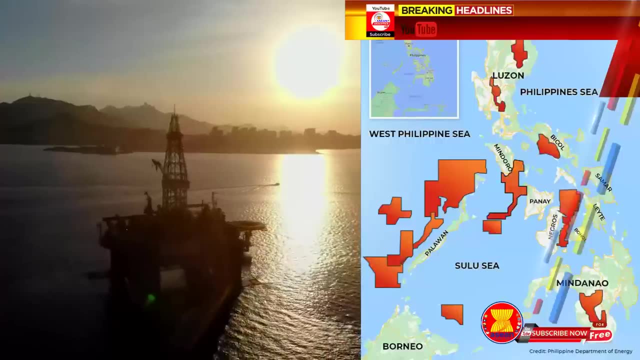 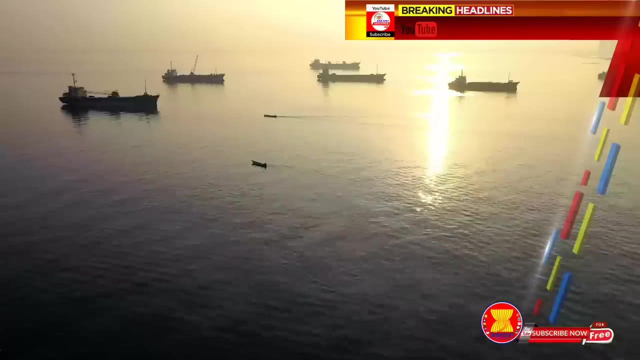 believed to be found inland in offshore waters, including those in the northern province of Cagayan, Ragay Gulf in Bicol, offshore Mindoro, the New Palawan Block, northern Cebu and the Cotabato Basin. These are the present and prospective oil fields in the country, as the Philippines is seeking to 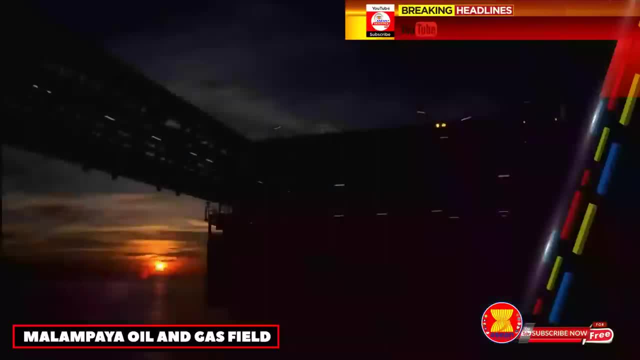 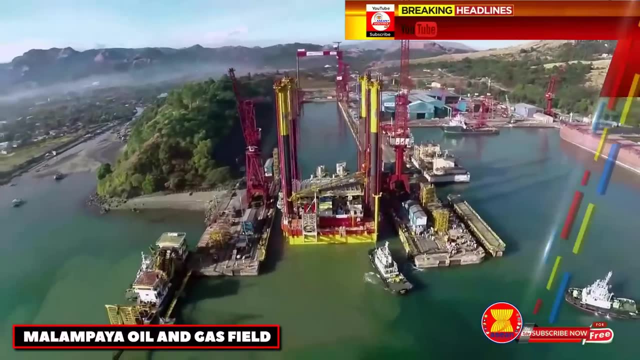 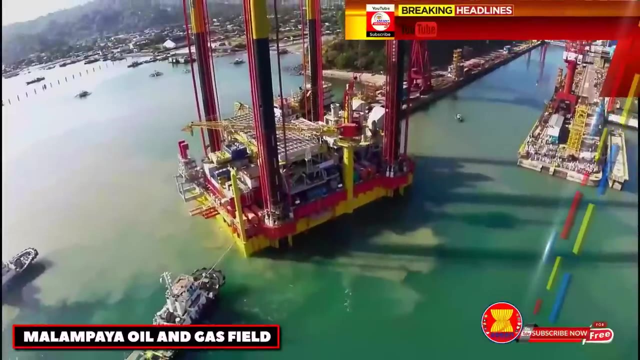 revive its moribund upstream oil industry. The Malampaya Oil and Gas Oil Field, 50 kilometers west of Palawan Island, has produced a total of 1.9 trillion standard cubic feet of gas as of the end of 2017 and 75 million barrels of natural gas liquids. It supplies five power plants in Luzon. 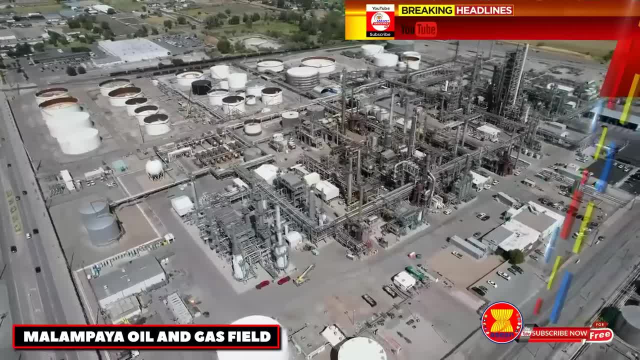 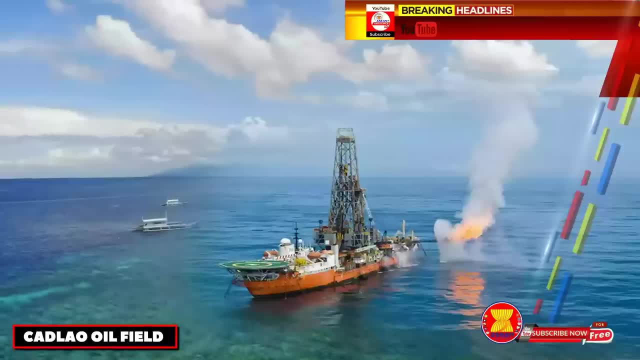 the country's largest island, with a combined capacity of 3,200 megawatts. Cadlao's oil field estimated recoverable volume of 3,200 megawatts. The oil field is the largest oil field in the country with volumes of 6.2 million barrels of oil are unlikely to have a huge impact on local 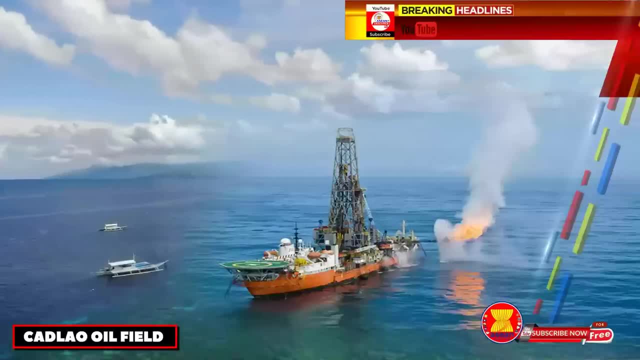 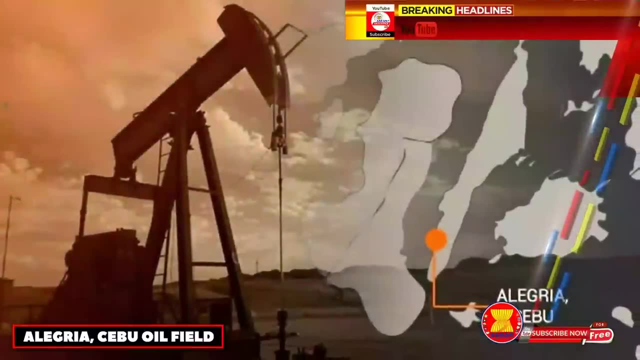 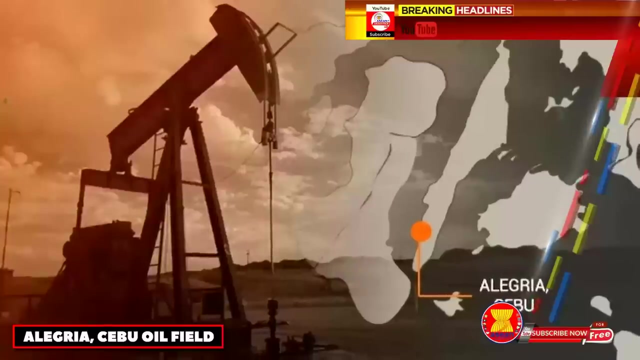 supply, But it will help minimize the import of petroleum products. Oil production could start by 2024.. In 2018, an estimated 27.9 million barrels of inland oil was discovered in Alegría Cebu by the Department of Energy and Service contractor China International Mining Petroleum Company. Limited, with an estimated 3.4 million barrels of recoverable oil. An estimated 9.4 billion cubic feet of natural gas reserves were found, with up to 6.6 billion cubic feet of recoverable gas, about 70 percent of the total estimated gas reserves. The Liguasen Marsh. 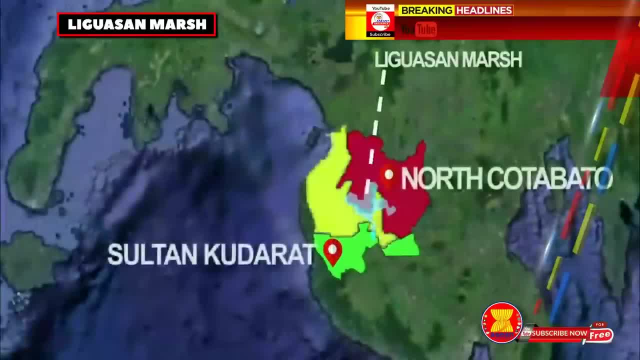 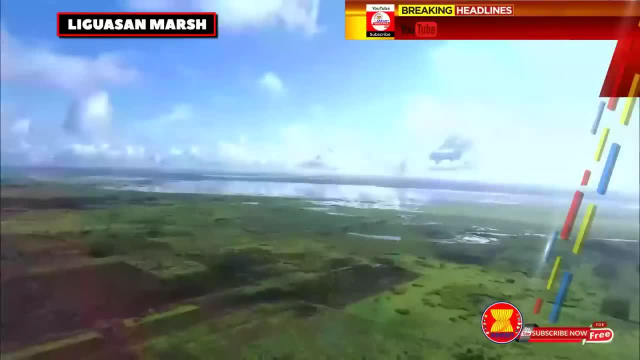 which covers 2,200 hectares straddling the provinces of Cotabato, Maguindanao and Sultan Kudarat, is estimated to hold 3.4 trillion cubic feet of natural gas and 4.8 billion barrels of.